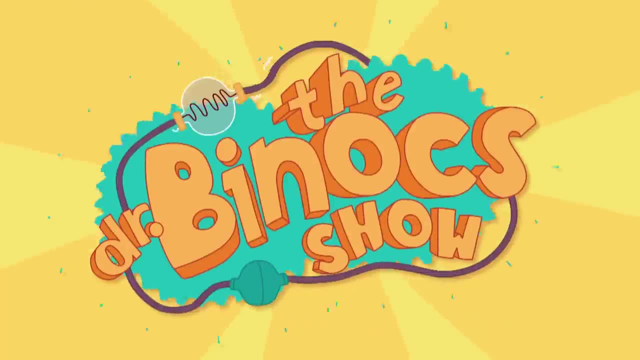 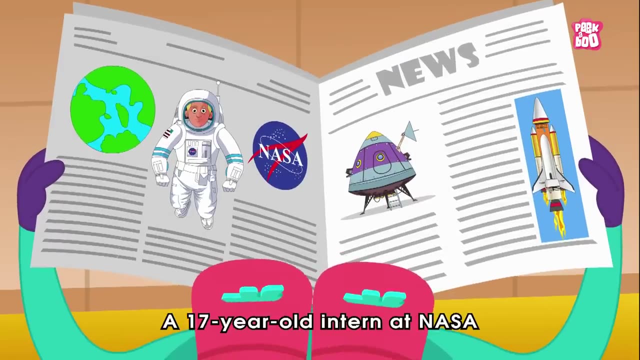 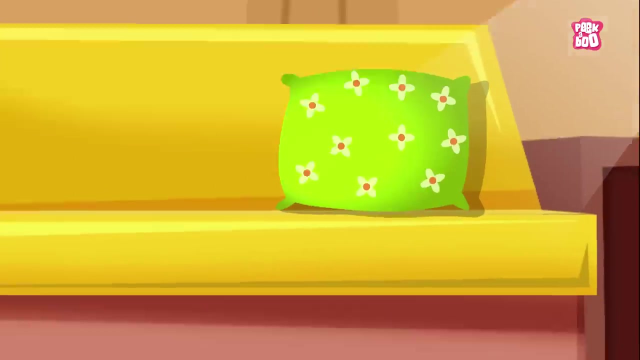 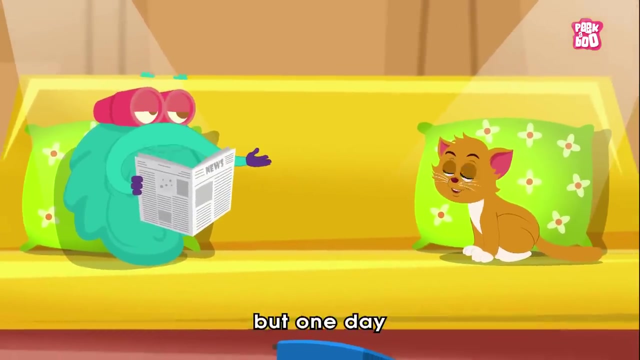 Hey Kitty, look, a 17-year-old intern at NASA has discovered a new Earth-like planet. Isn't that brilliant? Let's go there. I understand your curiosity, Kitty, But one day we might be able to settle on a different planet. 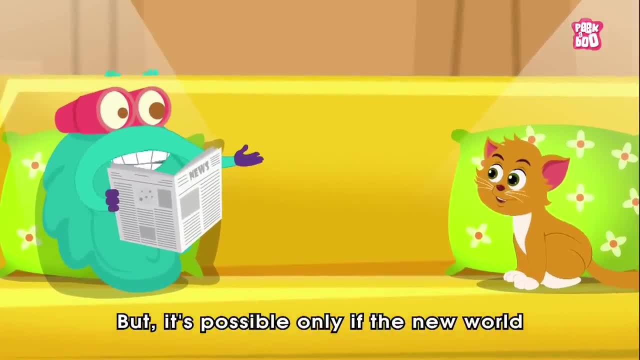 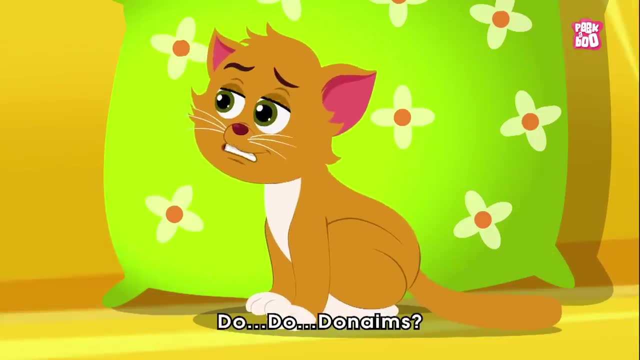 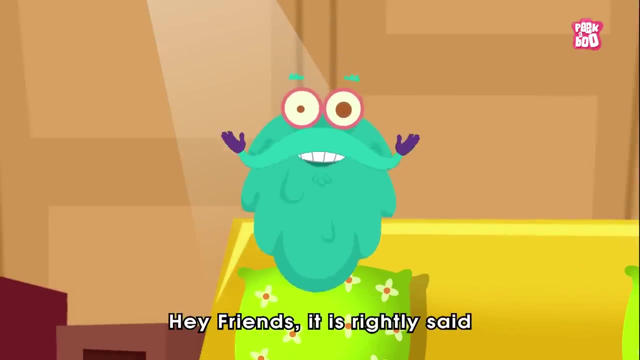 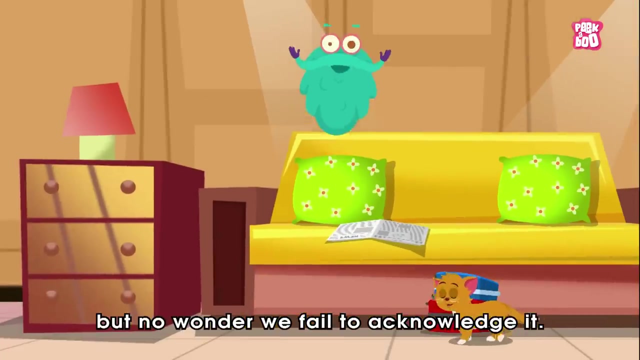 But it's possible only if the new world has all the four major domains of Earth present on it. It's domains Kitty, Hey, friends. it is rightly said that heaven is under our feet and over our heads, But no wonder we fail to acknowledge it. 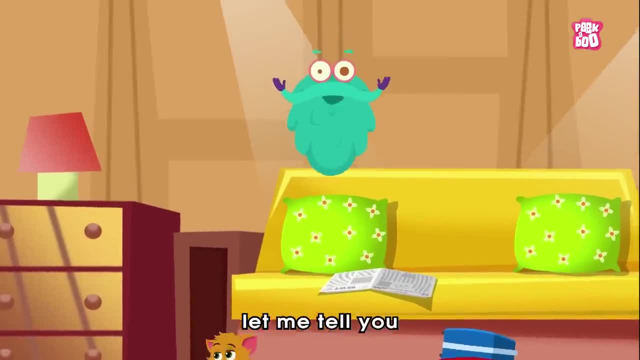 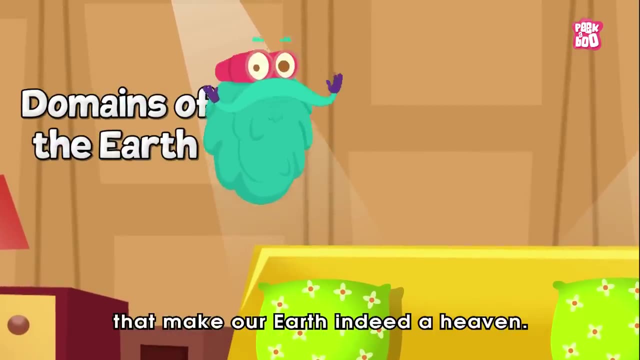 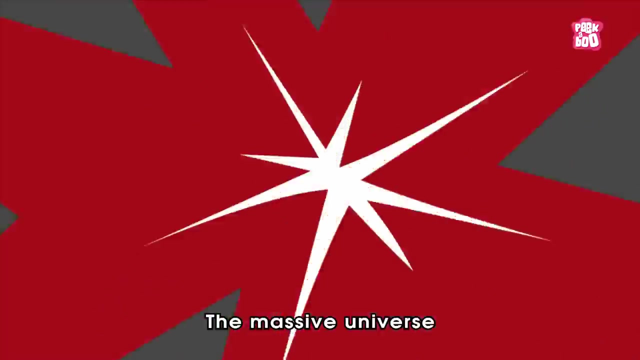 So in today's episode, let me tell you about those domains, Those four major domains of the Earth that make our Earth indeed a heaven. Zoom in. So what are the four domains of Earth? The massive universe formed millions of years ago has infinite undiscovered spaces. 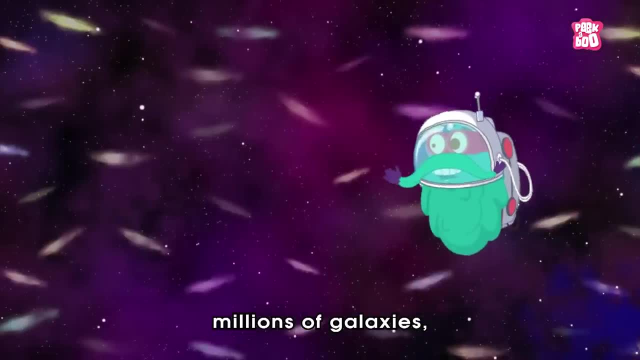 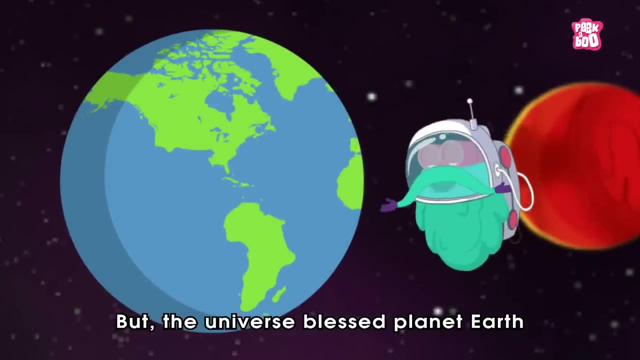 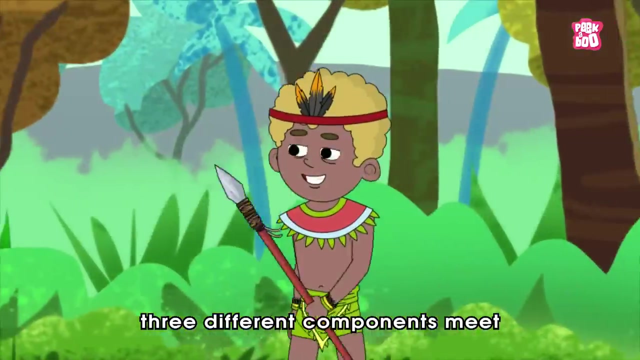 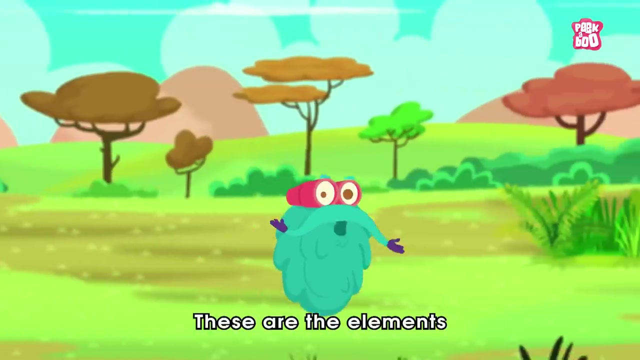 trillions of stars, millions of galaxies and the nine planets in our solar system. But the universe blessed planet Earth. The universe made the earth with living beings And to make life possible, three different components meet so humans can survive and thrive. These are the elements of land, water and air. 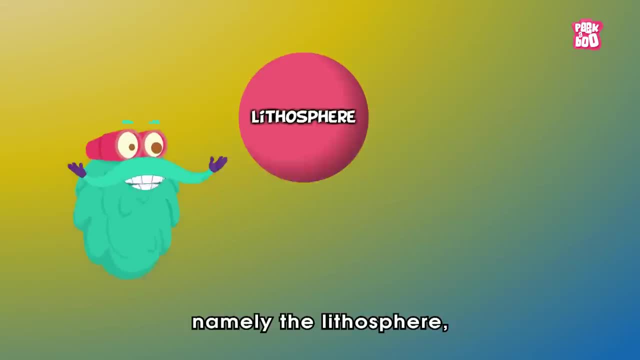 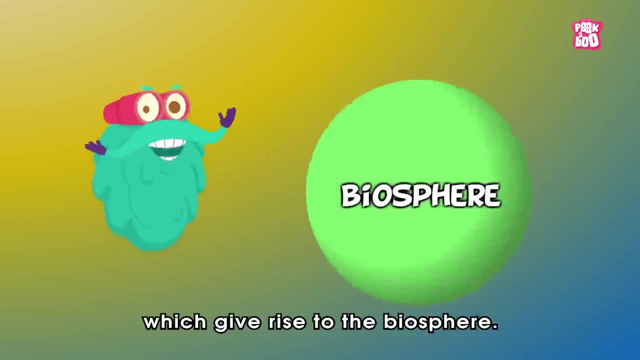 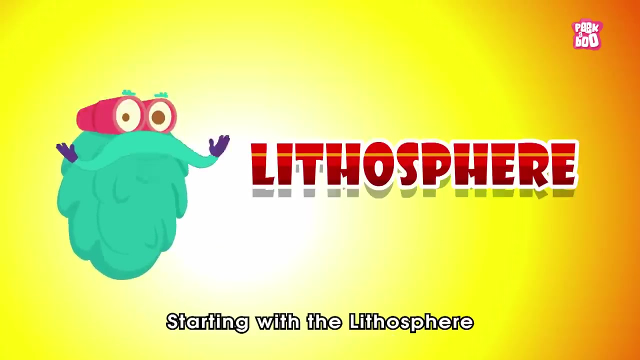 These are nothing but the domains of the earth, Namely the lithosphere, hydrosphere and atmosphere, Which give rise to the biosphere. Let's have a good look at each of them, Starting with the lithosphere, and to know about it, let's peek a little beneath the 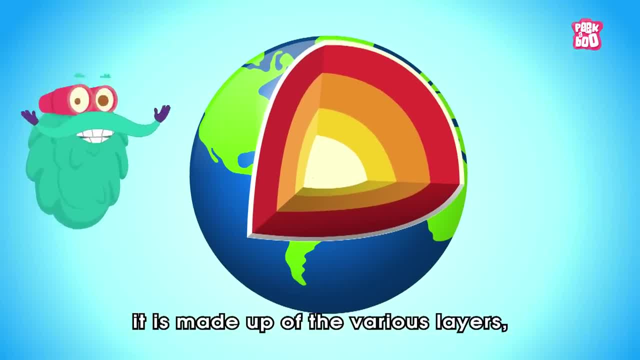 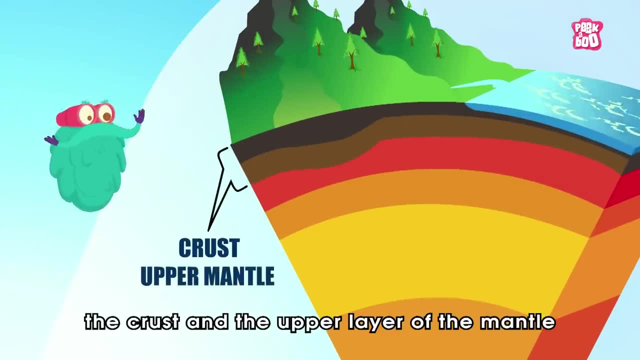 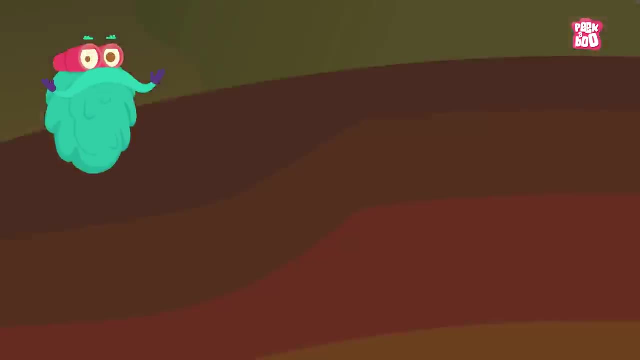 earth's surface. As you can see, it is made up of various layers, out of which the crust and the upper layer of the mantle make the lithosphere, which is basically the solid portion of the earth. The lithosphere is further divided into two parts. 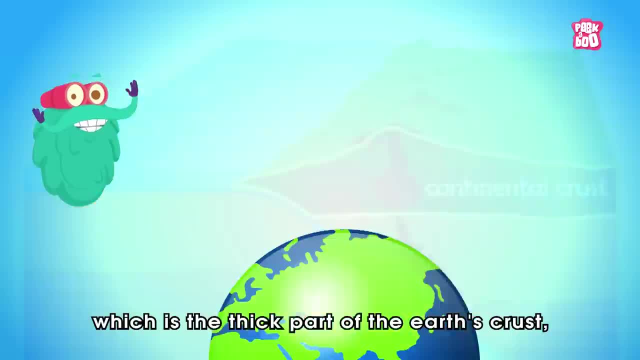 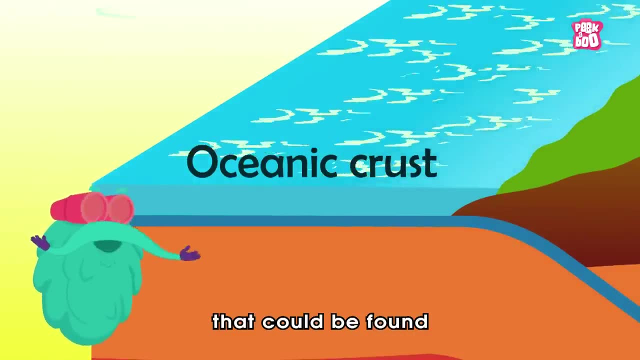 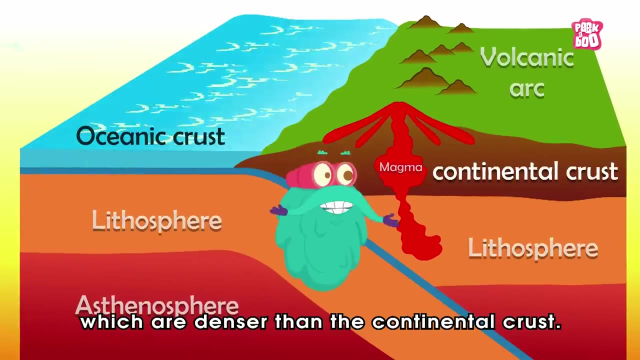 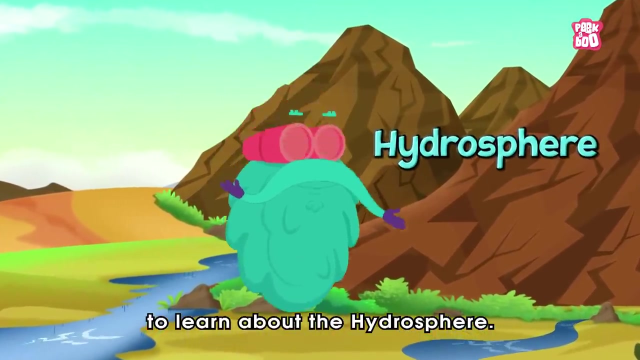 The continental crust, which is the thick part of the earth's crust, which forms the large land masses, and the oceanic crust that could be found deep under the ocean and seas which are denser than the continental crust. Now let us move further to learn about the hydrosphere. 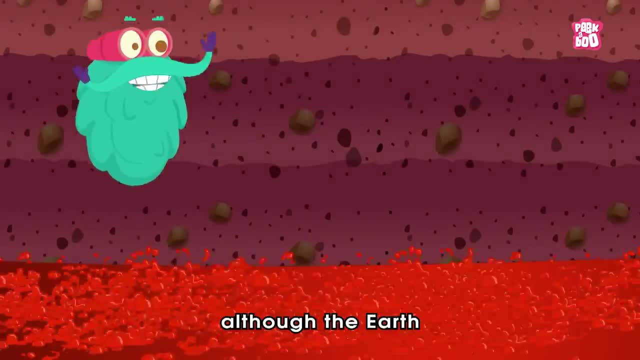 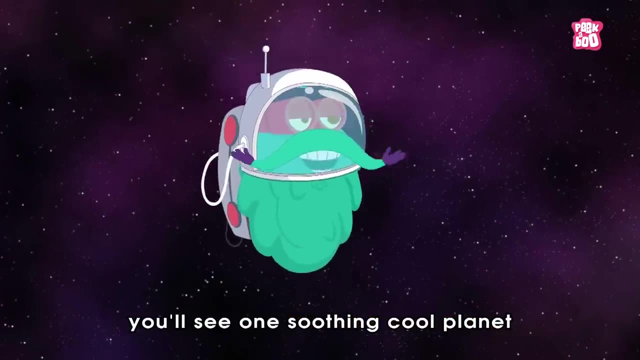 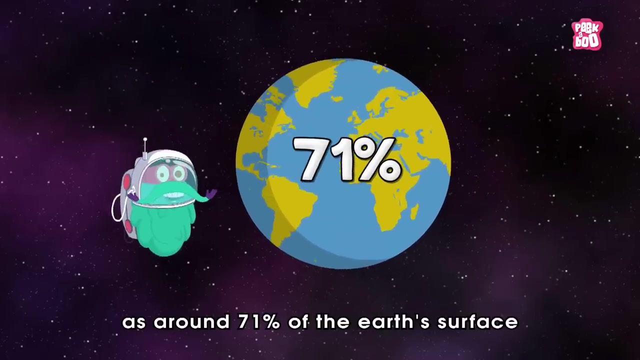 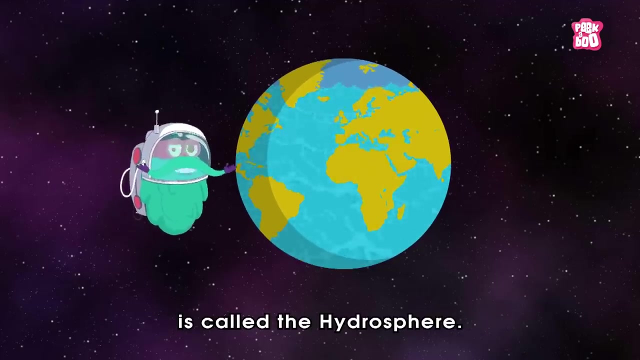 1. Hydrosphere. You see, although the earth seems hot and burning from inside, but when you look at it from space, you'll see one soothing, cool planet, due to its blue shade, as around 71% of the earth's surface is covered by water, and this water-covered area is called the. 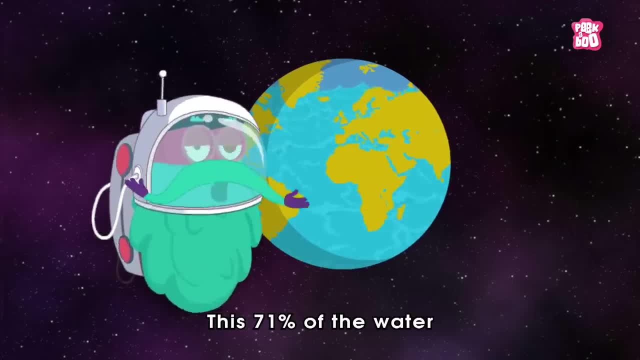 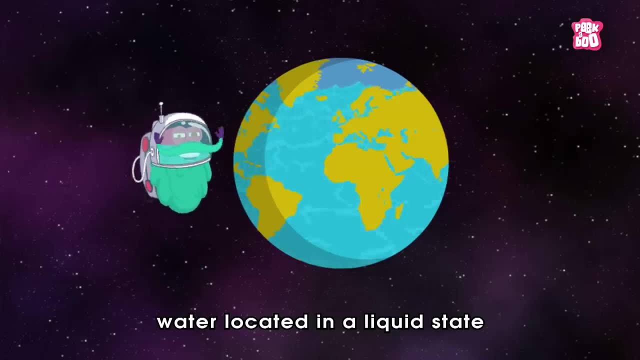 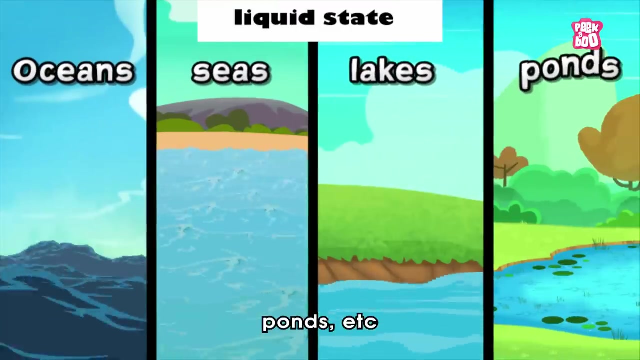 hydrosphere. This 71% of the water is found in three parts: 1. Hydrosphere: The hydrosphere consists of three different forms, ie water located in a liquid state into the water bodies such as oceans, seas, lakes, ponds, etc. in a solid state, such 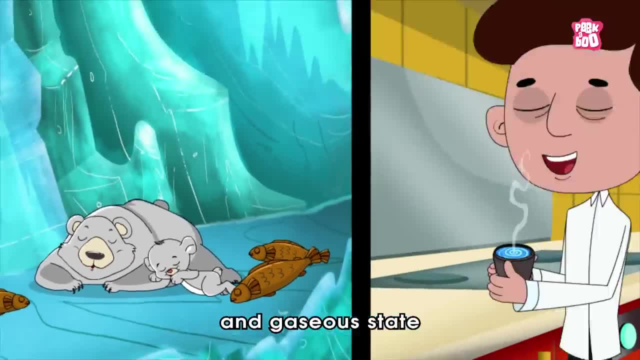 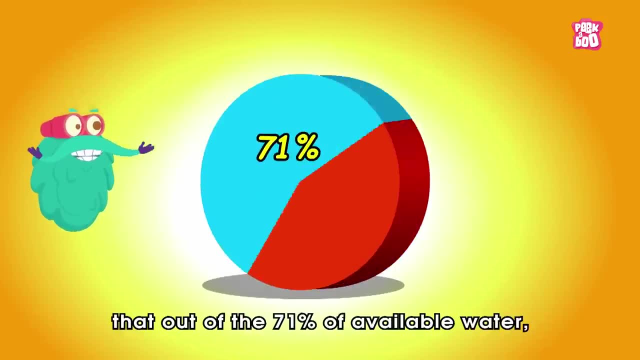 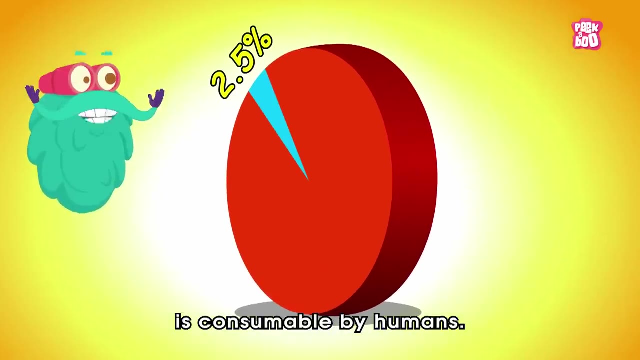 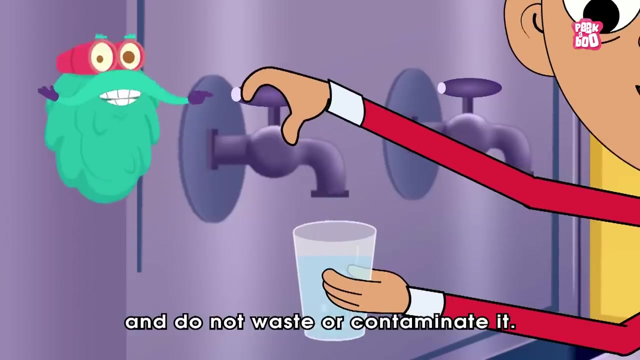 as ice and gaseous state such as water vapor, But always remember that, out of the 71% of available water, only 2.5% of the water is consumable by humans, So it is advisable that you consume water wisely and do not waste or contaminate it. 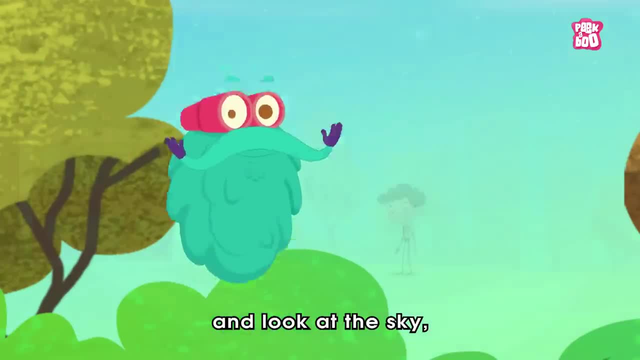 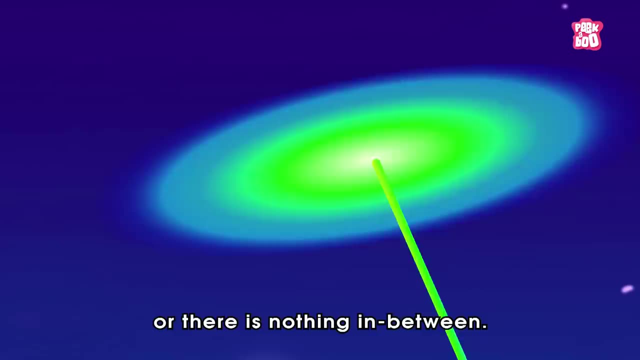 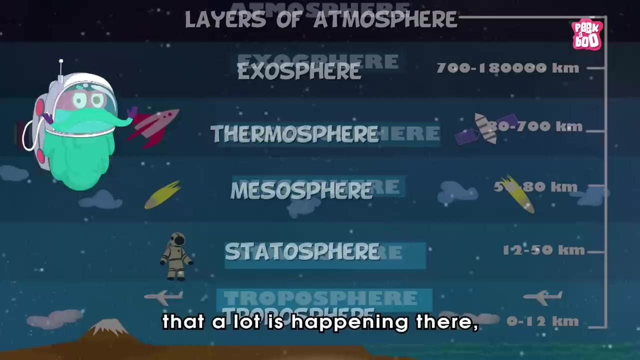 Now let us move further and look at the sky. I know you feel that the area between the surface of the earth and space is a vacuum or there is nothing in between, But let me inform you That a lot is happening there, as it is covered with a set of layers of gases we call the. 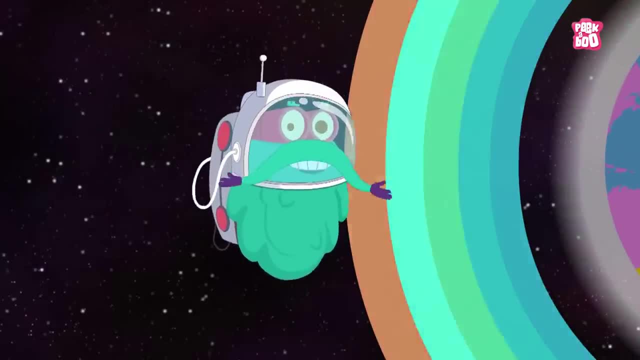 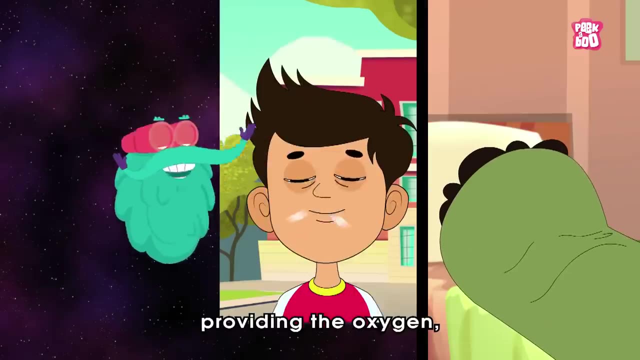 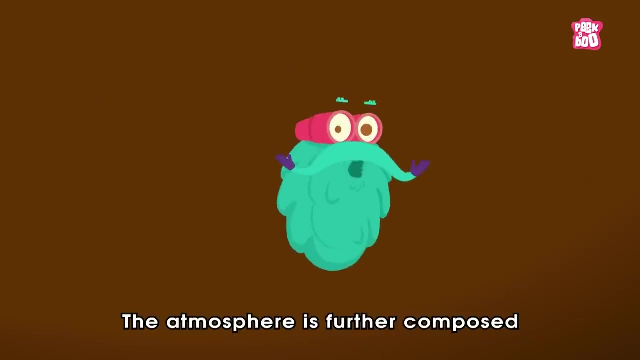 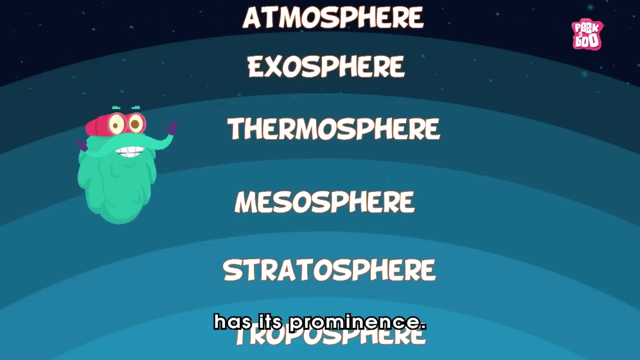 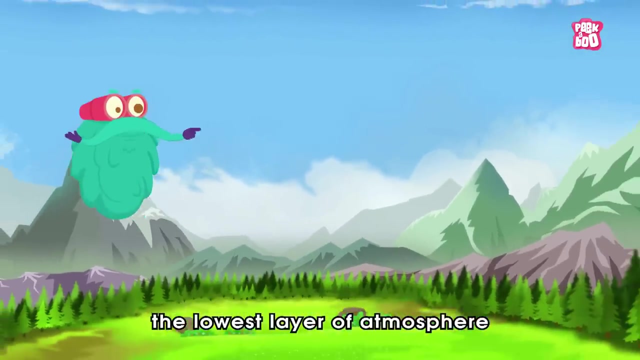 atmosphere that surrounds the earth. This invisible shield of gas performs various duties, like keeping us warm, providing the oxygen, and it is where the weather changes. The atmosphere is further composed of different layers: 2. And each layer has its prominence. The first layer is the troposphere, the lowest layer of atmosphere that ranges up to 5-9 miles. 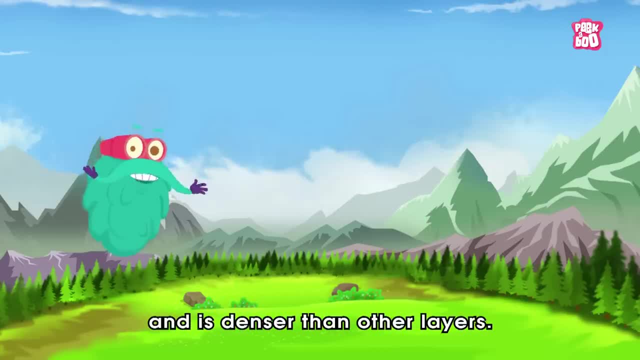 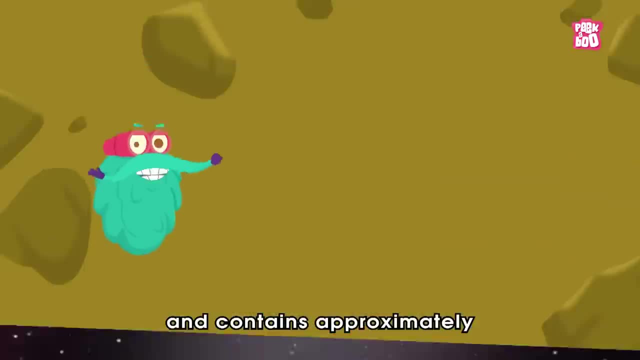 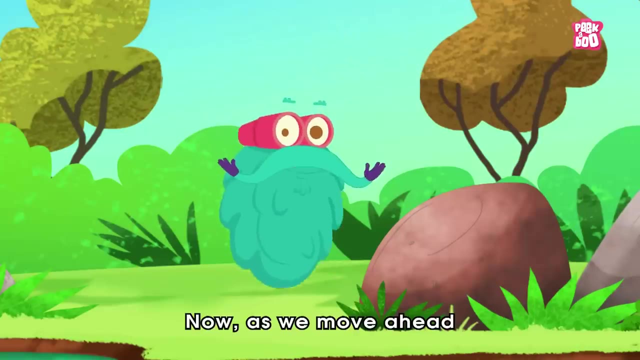 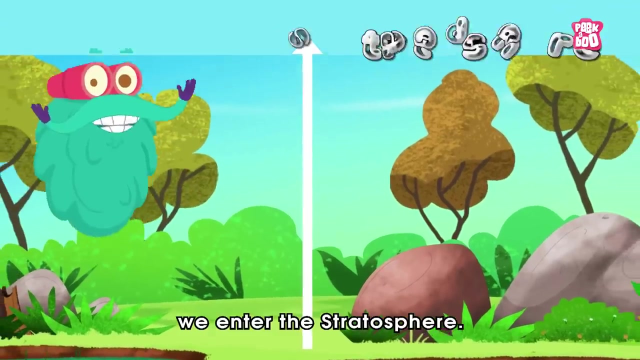 above the earth's surface and is denser than other layers. The troposphere is where all of earth's weather occurs and contains approximately 80% of the total mass of the atmosphere. Now, as we move ahead upto 31 miles from the earth's surface, we enter the stratosphere. 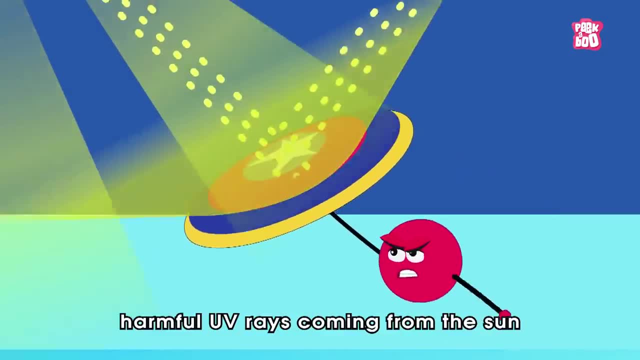 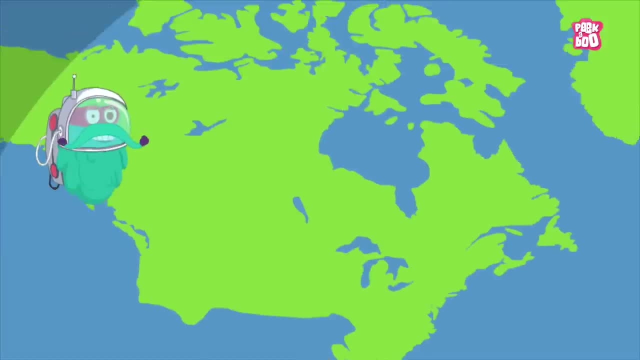 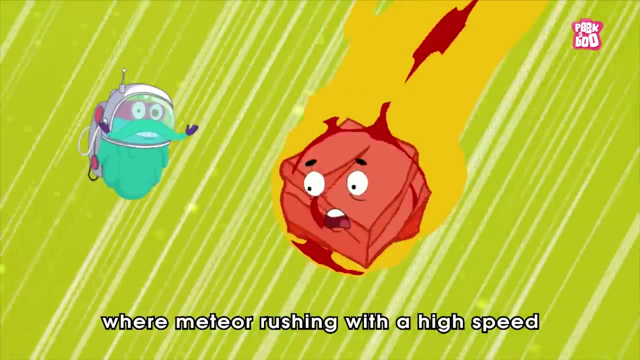 This vital layer absorbs harmful UV rays coming from the sun towards the earth with the help of the ozon layer present in it. 2. The next layer is mesosphere, where the meteors rushing with a high speed get burnt out. 3.. 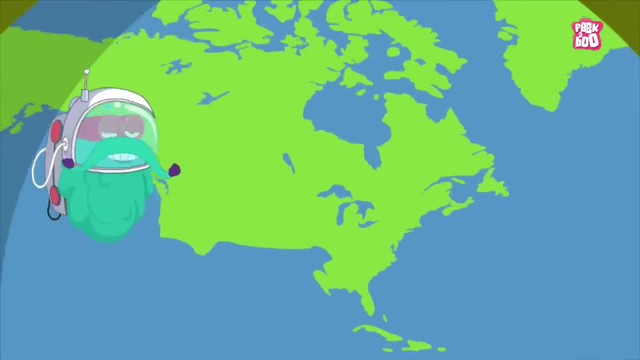 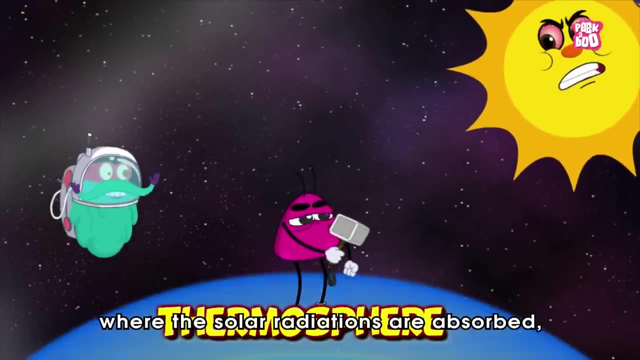 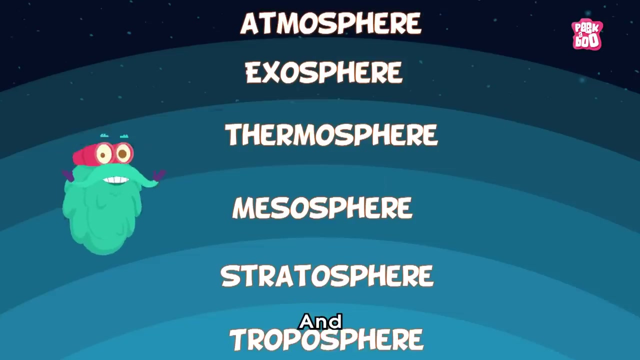 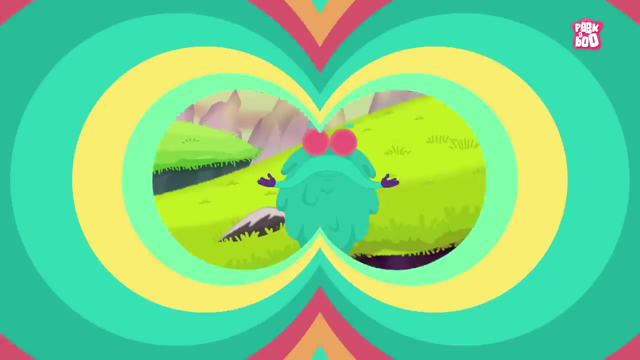 Let us take a look at the stratosphere. So it is a stratosphere, and after that comes the thermosphere, where the solar radiations are absorbed and you can witness the Aurora in the same layer. and the last layer is exosphere, which meets space. now coming back to the fourth domain of earth, that 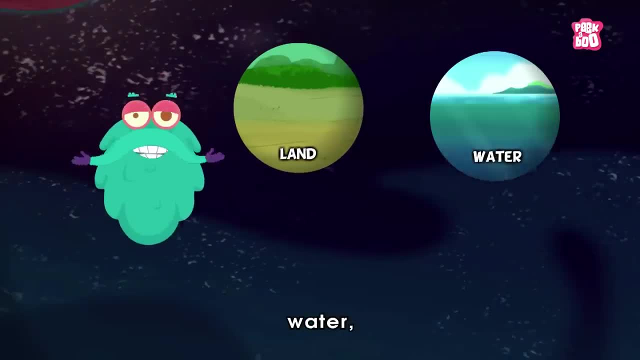 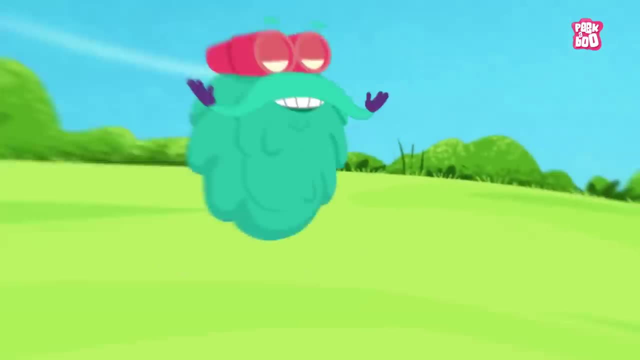 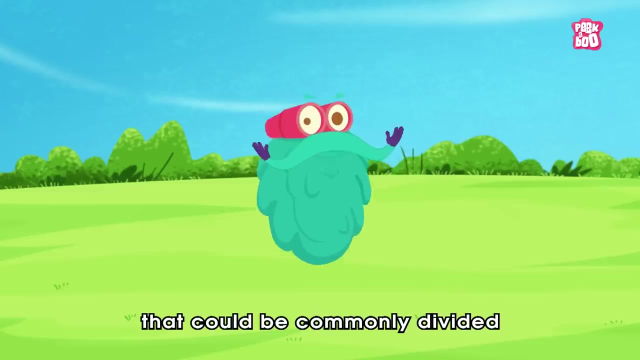 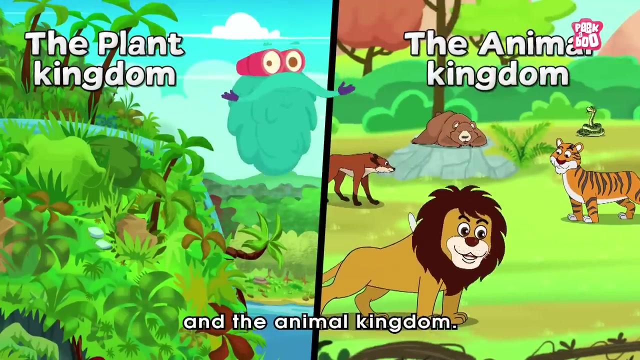 brings all the elements such as land, water and air together, is our last sphere, the biosphere. the biosphere represents every part of earth where living organisms are found. that could be commonly divided into two main parts: the plant kingdom and the animal kingdom. this sphere ranges from the vast sky to